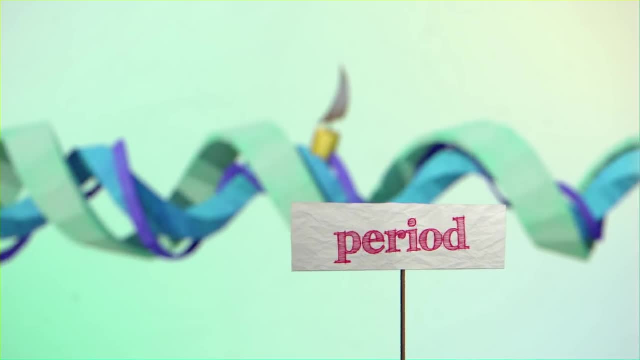 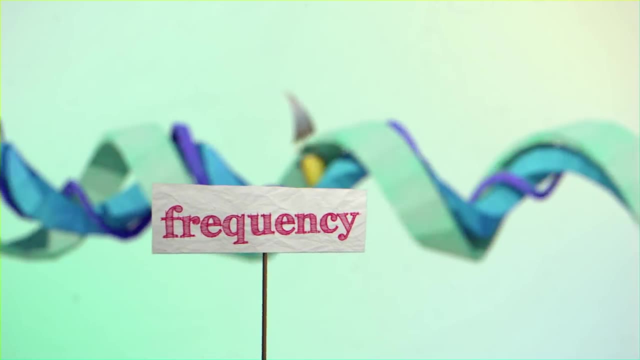 on. That is how long it takes a wave to go through its full range of motion. once The same information can be expressed in a different way by calculating the wave's frequency. Frequency, as the name suggests, tells you how frequent the waves are, That is, how many. 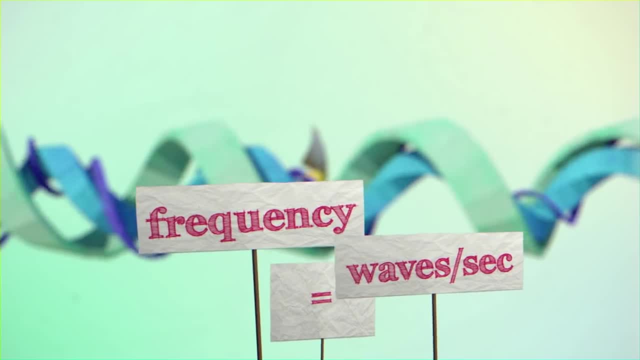 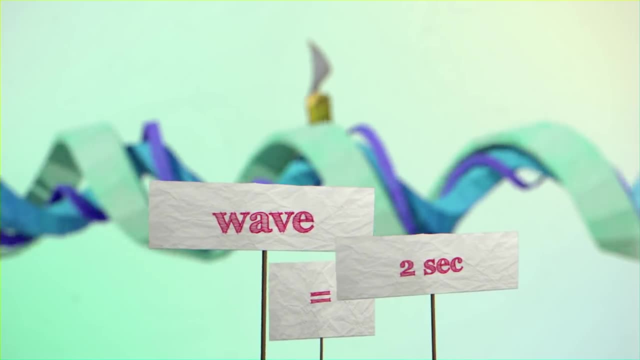 of them go by in one second. If you know how many seconds one full wave takes, then it's easy to work out how many waves go by in one second. In this case, since each wave takes two seconds, the frequency is 0.5 waves per second. 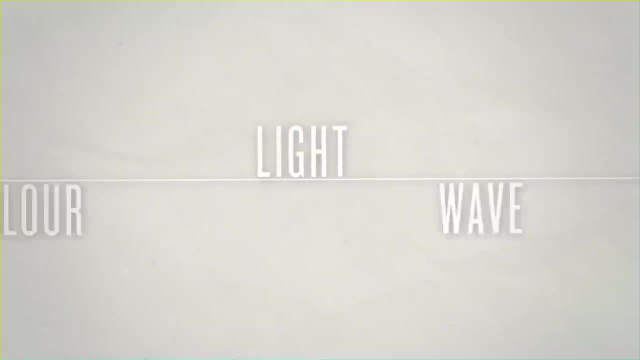 So enough about bobbing corks. What about light and colour? If light is a wave, then it must have a frequency, right? Well, yes, it does, and it turns out that we already have a name for the frequency of the light that our eyes detect: It's called colour. 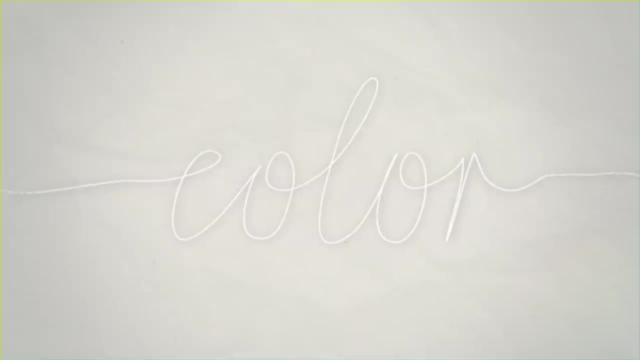 That's right. colour is nothing more than a measure of how quickly the light waves are waving. If our eyes were quick enough, we might be able to observe this periodic motion directly, like we can with the cork in the ocean. The frequency of the light we see is so high: it waves up and down over 400 million million. 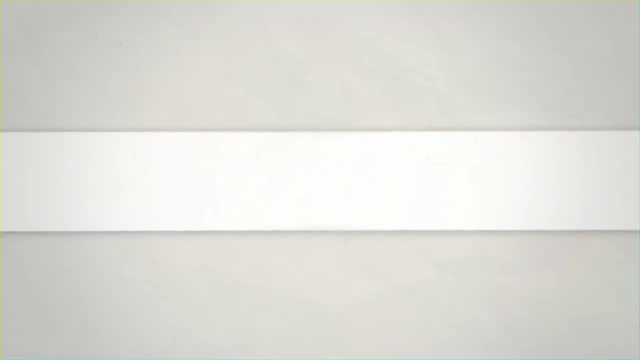 times a second that we can't possibly see it as a wave, But we can tell by looking at its colour what its frequency is. The lowest frequency light that we can see is red and the highest frequency is purple. In between, all the other frequencies form a continuous 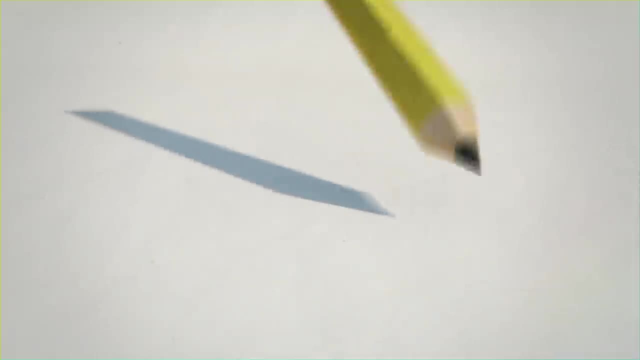 band of colour called the visible spectrum. So what if you had a yellow pencil sitting on your desk? Well, the sun emits all colours of light, so light of all colours is hitting your pencil. The pencil looks yellow because it reflects yellow light more than it reflects. 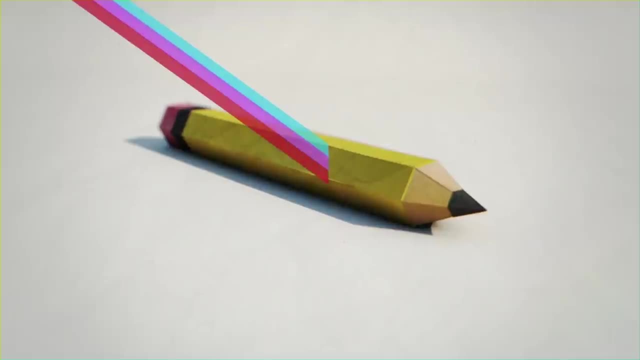 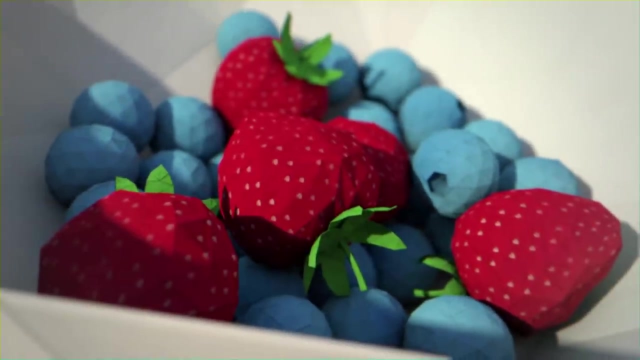 the other colours. What happens to the blue, purple and red light? They get absorbed and the energy they are carrying gets turned into heat. It's similar with objects of other colours: Blue things reflect blue light, red things reflect red light, and so on. White. 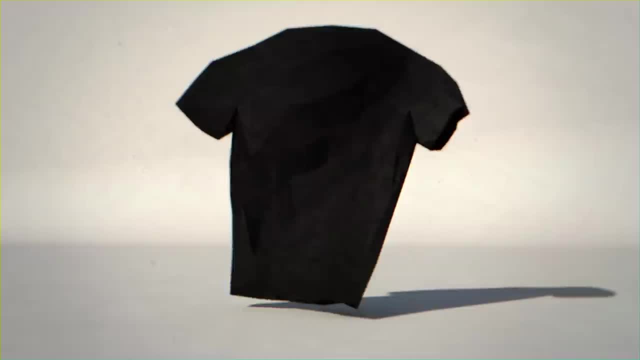 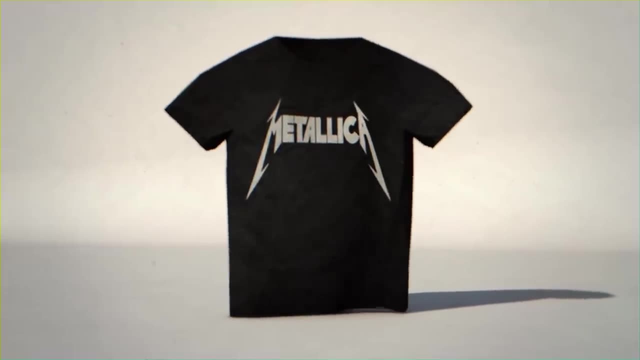 objects reflect all colours of light, while black things do exactly the opposite and absorb at all frequencies. This, by the way, is why it's uncomfortable to wear your favourite Metallica t-shirt on a sunny day. Subtitles by the Amaraorg community.